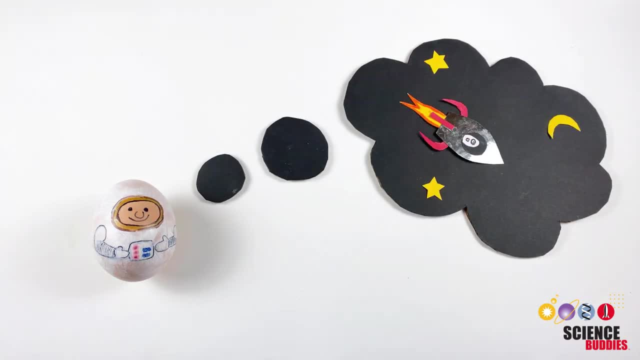 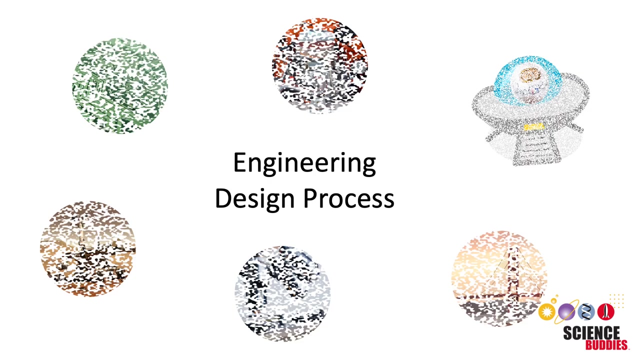 Our Eggstronaut is ready for its next adventure. However, before takeoff, it still needs a way to safely land on a new planet. How can we solve this problem? We can use the engineering design process to design and build products, like building an egg drop lander to help protect. 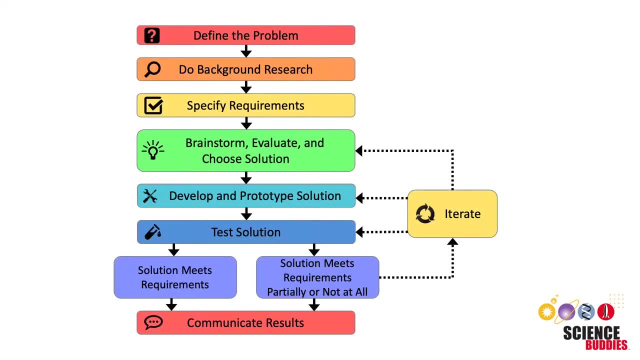 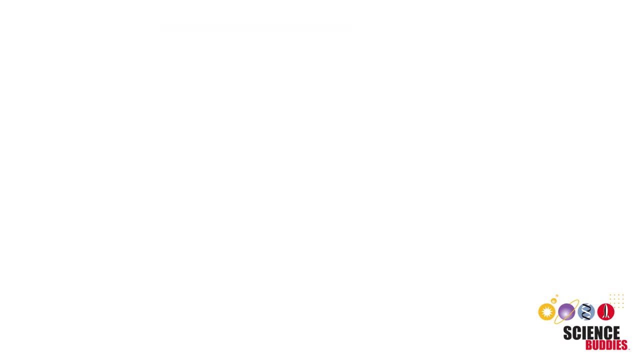 our Eggstronaut. The engineering design process has several steps. Let's look at each step as we design and build an egg drop lander for our Eggstronaut. The first step is to define the problem that needs to be solved. A good way to define a problem is to answer the following. 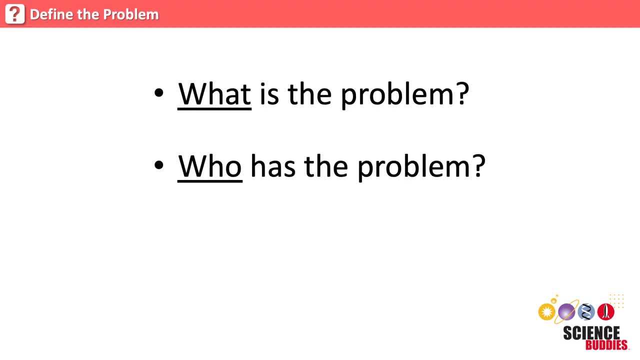 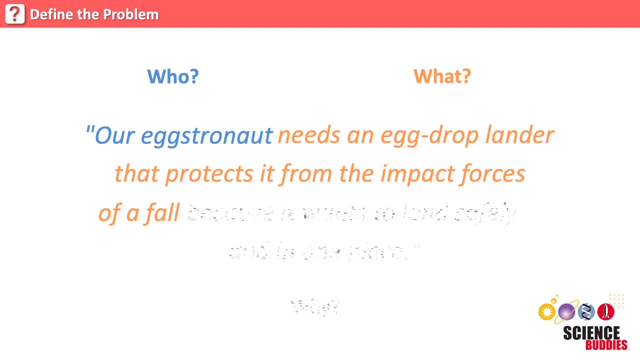 questions. What is the problem? Who has the problem And why is the problem important to solve For our egg drop lander project? the problem statement might be: our Eggstronaut needs an egg drop lander that protects it from the impact forces of a fall, because it wants to land safely. 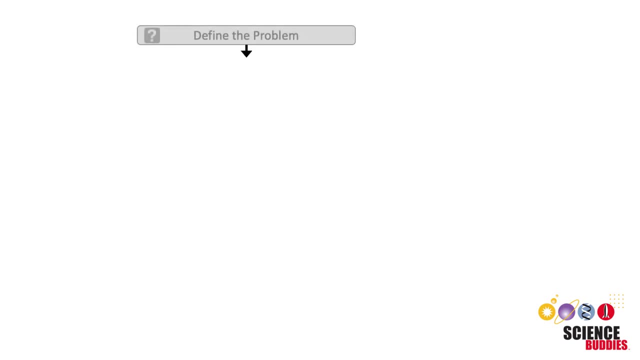 and safely from the impact forces of a fall, because it wants to land safely and safely from our Eggstronaut and in one piece. Now that we know exactly what problem we need to solve, we can move on to step two, which is doing background research. In this step, we want to find out as much as possible. 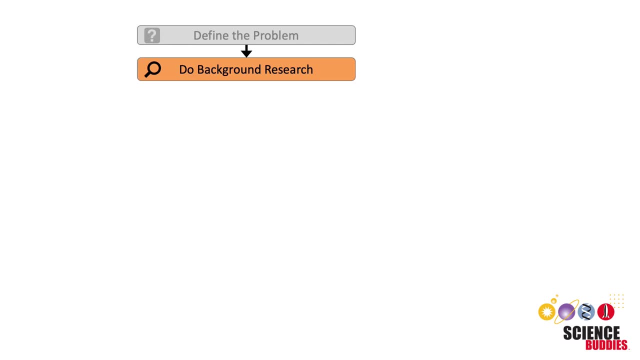 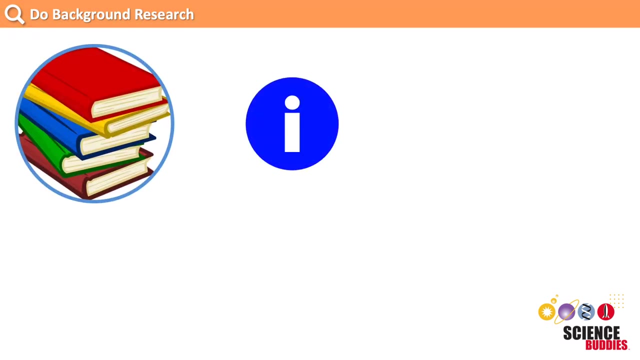 about our problem and learn from the experiences of others. When doing background research, we can find information in many different places. We can use books in the library, search the internet or ask an expert or specialist questions about the problem we are trying to solve. Learning more about the problem often sparks initial ideas for how to 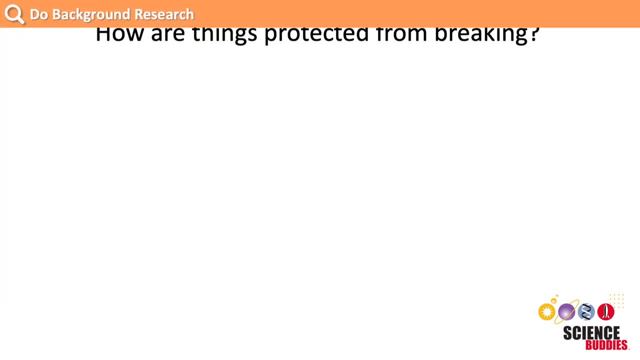 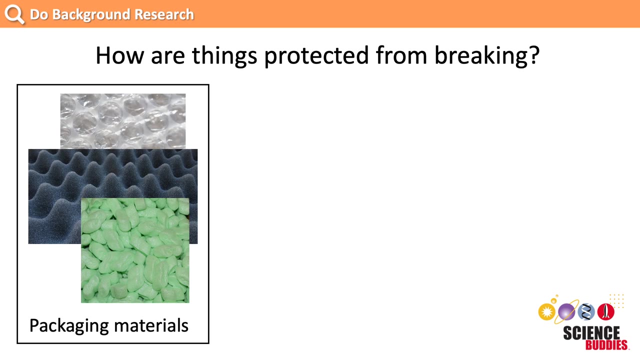 solve it. To get ideas for our egg drop lander, let's find out how things are usually protected from breaking. After doing some research, we find three common solutions used by others that may be helpful in designing our solution. First, we find that packaging materials like foam, bubble wrap. 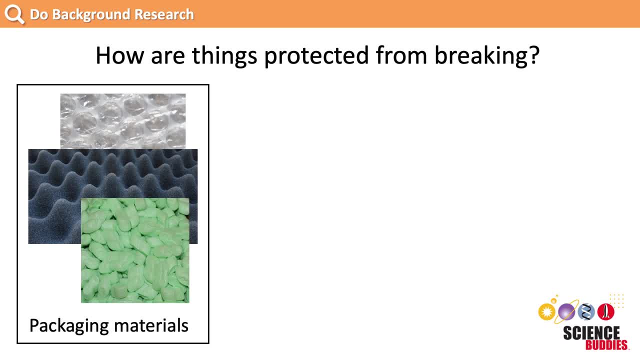 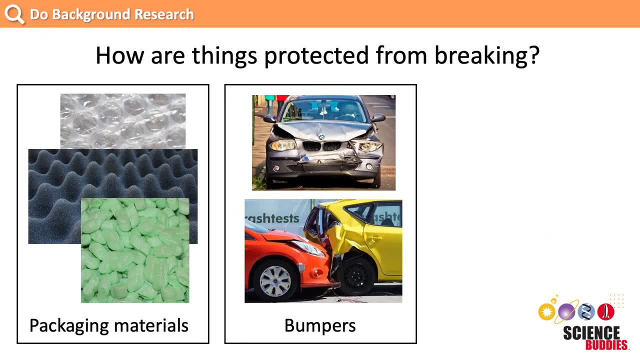 or packing peanuts protect objects during shipment by absorbing energy from bumps and drops that could otherwise cause an object to break. Similarly, we find that car bumpers are designed to crumple in order to absorb some of the energy from a head-on car collision. This helps. 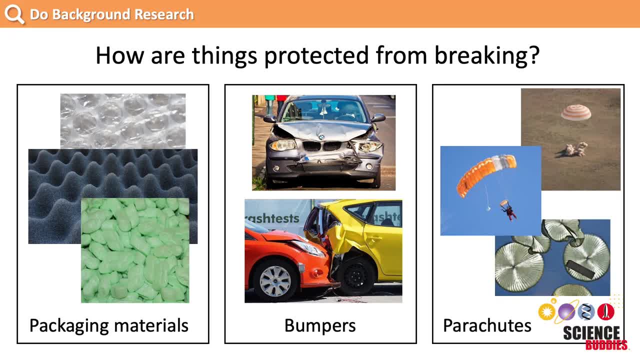 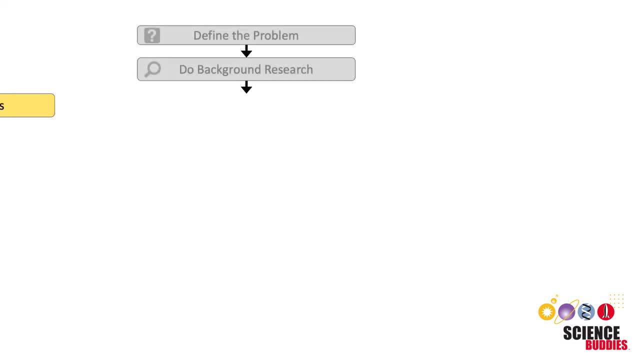 keep the people inside the car safer. We also find that parachutes are used to slow down people, spacecraft and cargo to help them land with less force. This is all useful information that we can use when designing our egg drop lander. The next step is to specify the requirements for our design. To do that, we need to think. 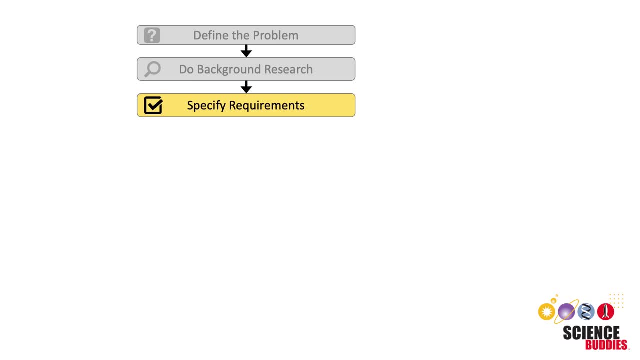 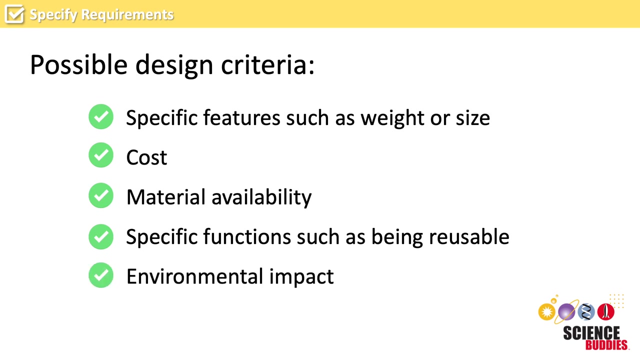 about what criteria our design must meet in order to be successful. Such design criteria might include specific physical features, such as weight or size, cost, material availability, specific functions, such as being reusable, environmental impact and many more. What are some criteria that? 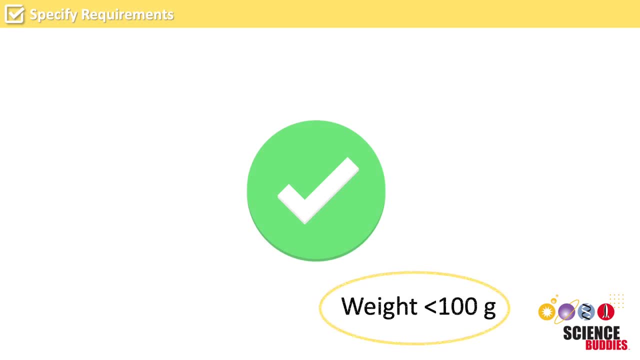 our egg drop lander needs to meet. It needs to be lightweight or weigh less than 100 pounds. It needs to be smaller than 20 centimeters in length, width and height. It needs to be made from inexpensive materials. It needs to protect our extra knot from breaking when falling from. 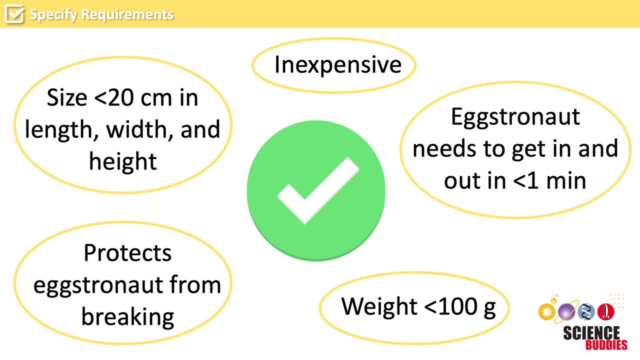 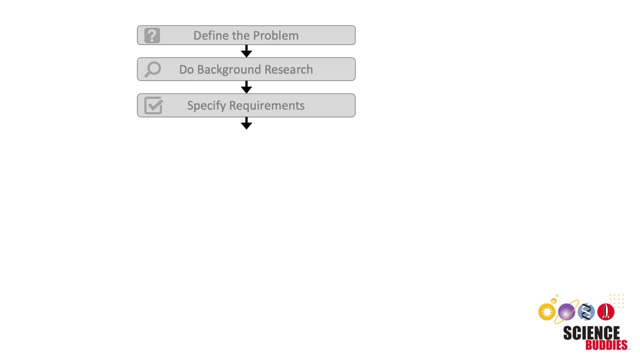 eight feet, And the extra knot needs to be able to get in and out of the lander in less than one minute. With these design criteria and the information from our background research in mind, we can now start step four: brainstorming and evaluating possible solutions for our problem. 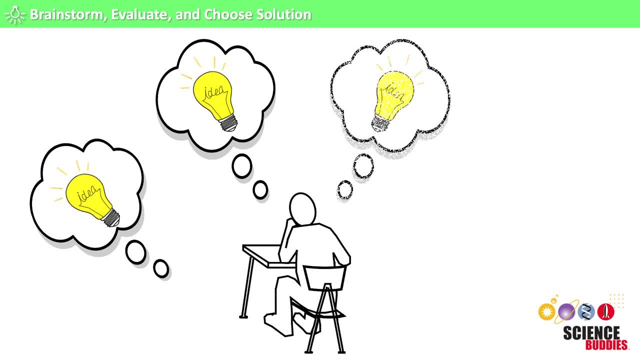 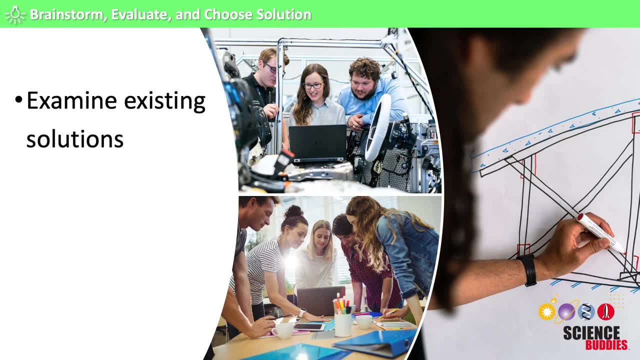 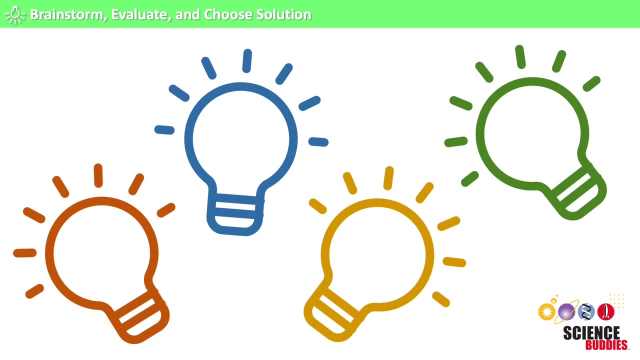 At this point, we want to come up with as many solutions as possible, even wild and crazy ones that may not work. This step often includes examining existing solutions, brainstorming new ideas and making sketches of possible designs. How could we design our egg drop? 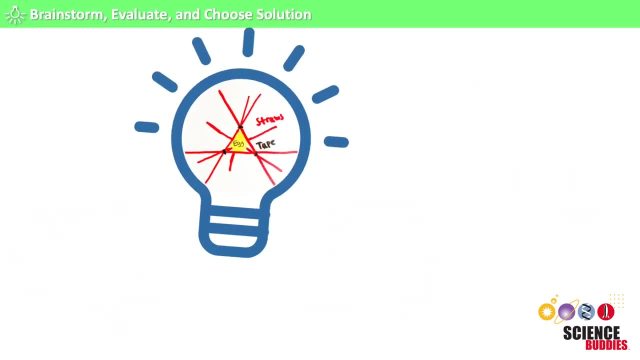 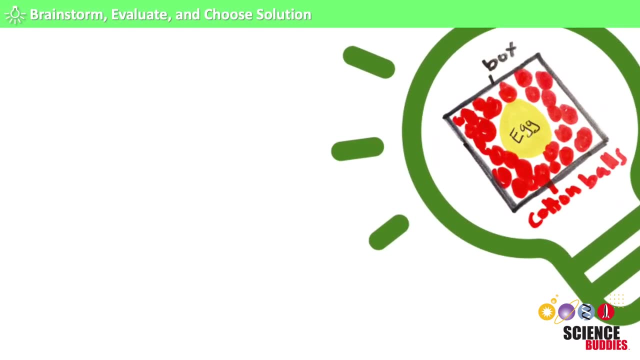 lander. Some ideas are: we could use straws to build lots of bumpers that create a crumple zone around our extra knot. We could create a box with lots of foam, cotton balls or bubble wrap cushioning that protects our extra knot. We could build a parachute that. 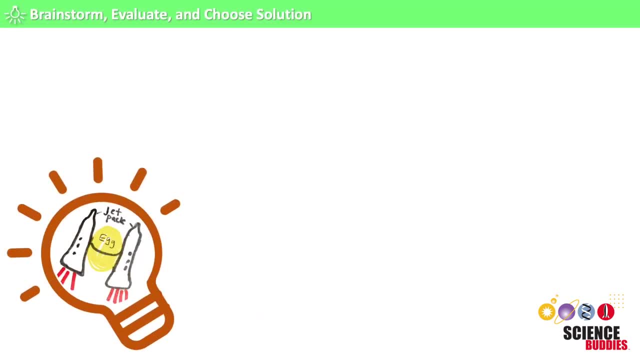 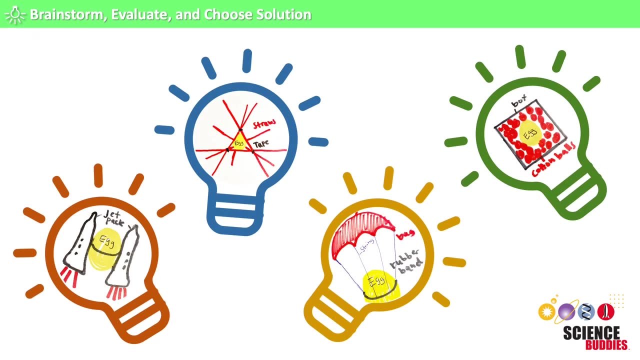 slows down our extra knot's fall. Or we could use a jet pack with thrusters to gently land our extra knot on the ground. These are all good ideas. How do we choose which solution to try? First, we eliminate any that do not fit the design criteria we identified in step three of the 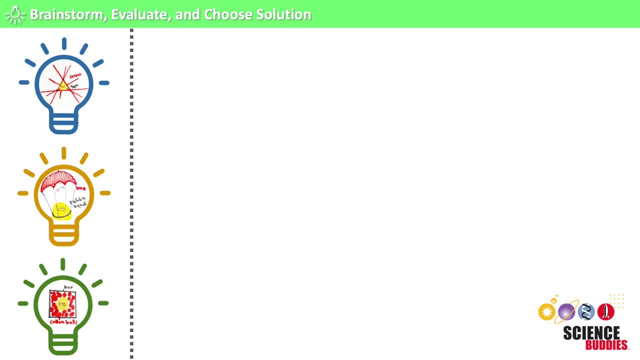 engineering design process. Then we evaluate the designs that are left. To help you evaluate your design: you need to know which design is the best fit for you. You need to know which design is the best fit for you. You need to know which design is the best fit for you. You might try these. 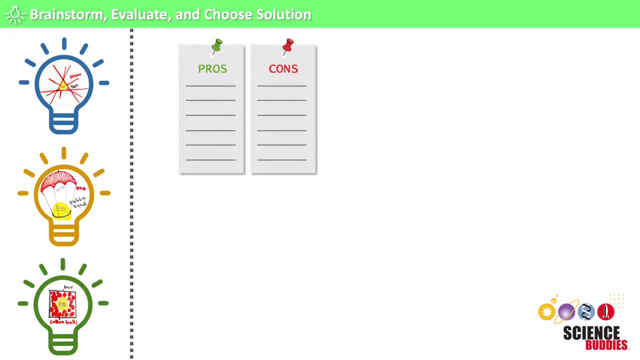 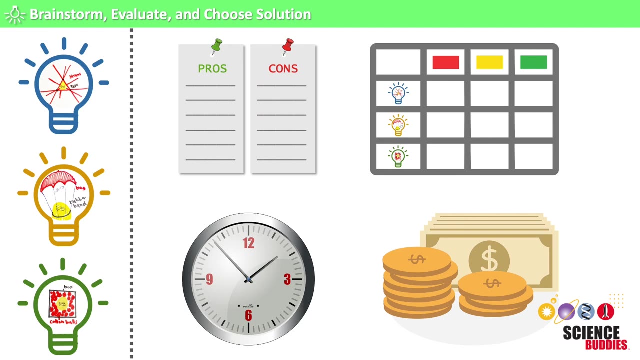 strategies. Make a pros and cons list for each design, Figure out which design meets the most design criteria, Compare how long it would take to build each design and determine how much each design will cost to build. During this process, it may be obvious which solution to try: first Or 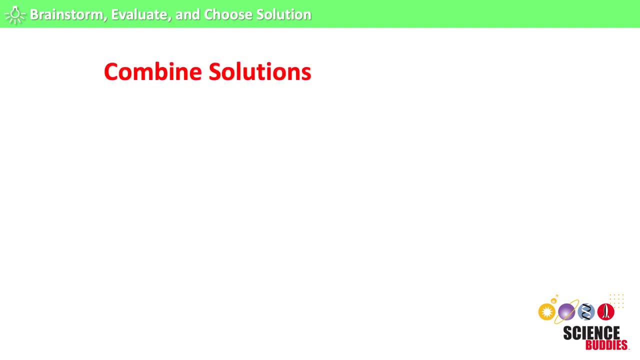 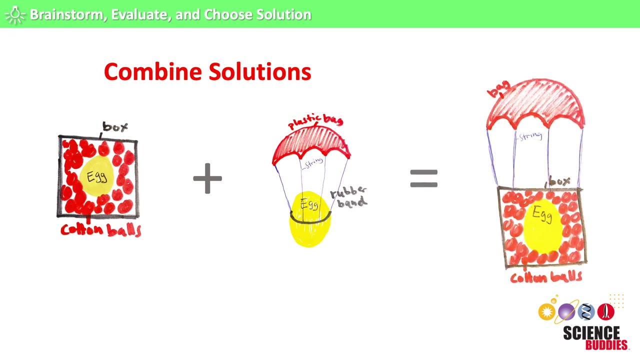 it may make sense to combine several solutions to make an even better solution. For example, to build the best possible egg drop lander. we could combine two of our ideas from brainstorming and make a box with both cushioning to protect the extra knot and a parachute to slow down the box's fall. 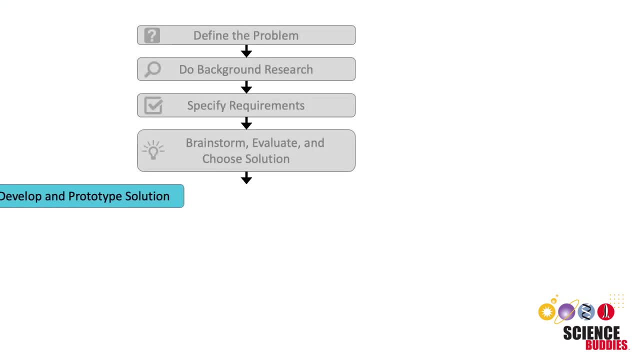 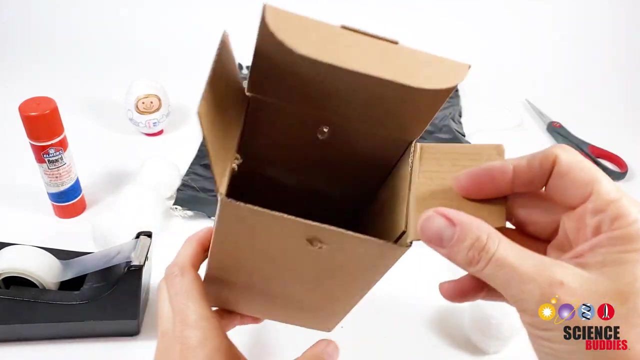 Once a solution has been selected, it is time to start developing and prototyping the chosen design. Making a prototype means making a working model of our solution. This is a key step in the development of a final solution. To build our prototype egg drop lander, we will take the box. 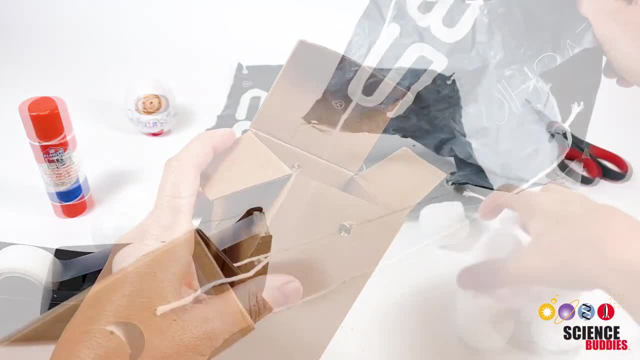 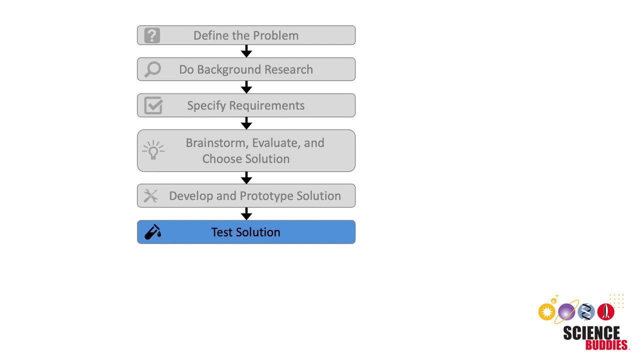 that holds our extra knot and place it on top of the box that holds the box that holds the box that holds our extra knot, add some cushioning and then attach a parachute. The next step is to test the prototype. Testing allows us to find out if our solution works and how well the prototype meets. 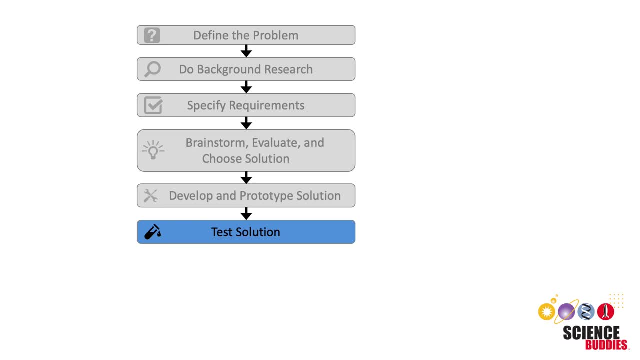 all of the design criteria. Testing almost always involves collecting data about the product's performance. It might also include getting feedback from others. Sometimes, test data will show that the solution does not meet all of the criteria yet. That is okay If that happens. 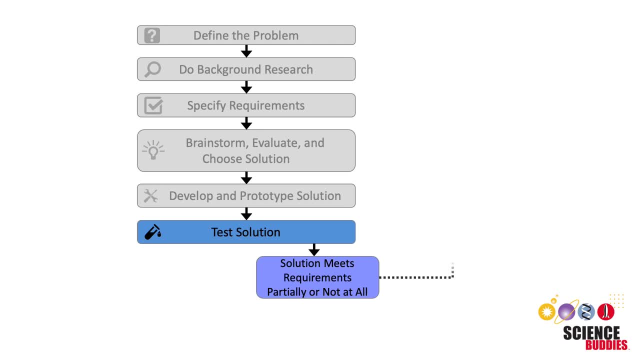 the project is not over. Instead, a loop starts that includes making changes to the design or trying a new design, testing the new solution, finding more problems and improving the design again. This process is called iteration. It is common to go through multiple iterations and 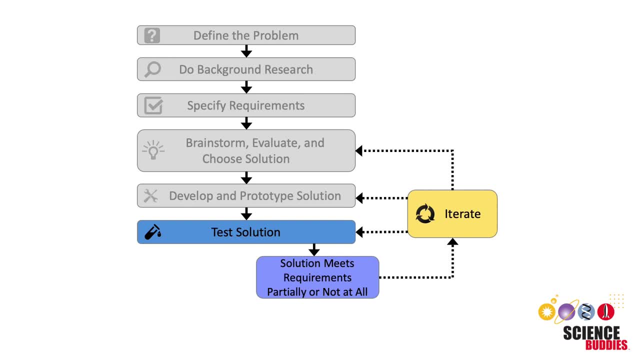 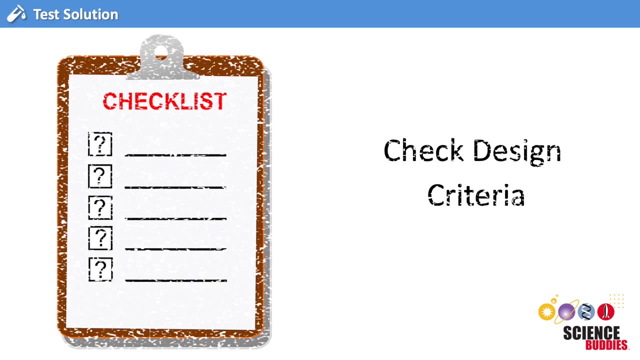 redesigns before arriving at a final solution that meets all the design criteria. How successful is our egg drop lander prototype? To find out, we need to check all the design criteria we listed earlier. We measure the weight and the size of the prototype. 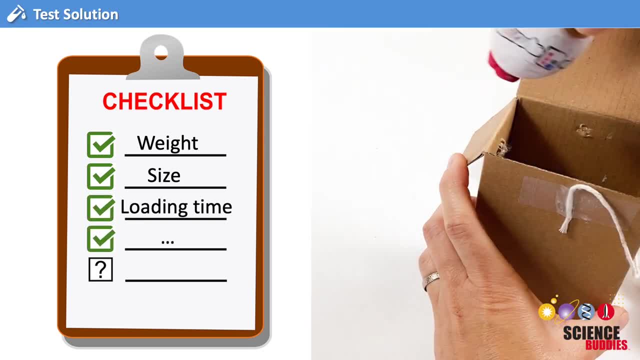 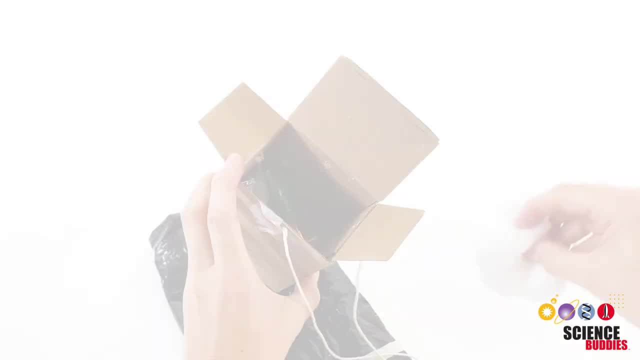 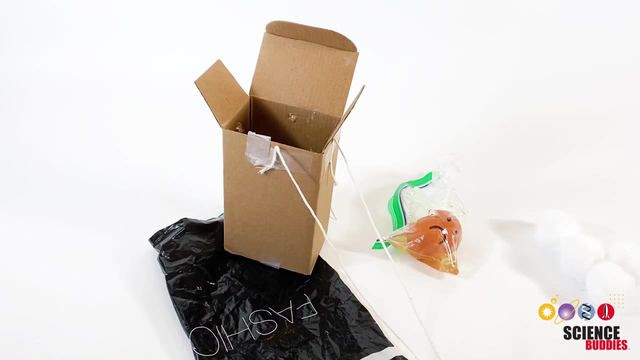 we test how long it takes for the extra knot to get in and out of the lander and, most importantly, we need to test if the egg drop lander protects our extra knot from breaking when dropped from eight feet. Oops, It looks like our solution doesn't work, Based on the results of our test.